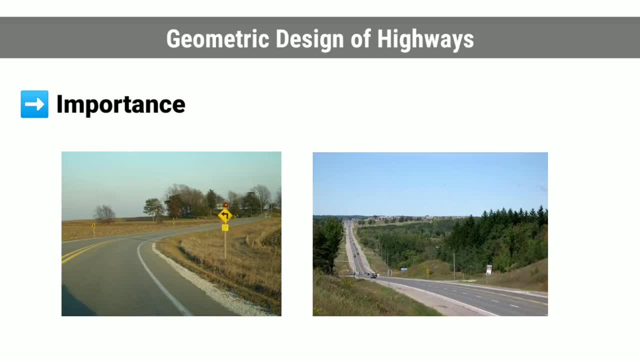 road during the initial alignment itself, taking into consideration the future growth of the traffic flow and possibility of road being upgraded to a higher category or to a higher design speed standards at a later stage. Now let's see. the geometric design of highway deals with following elements: 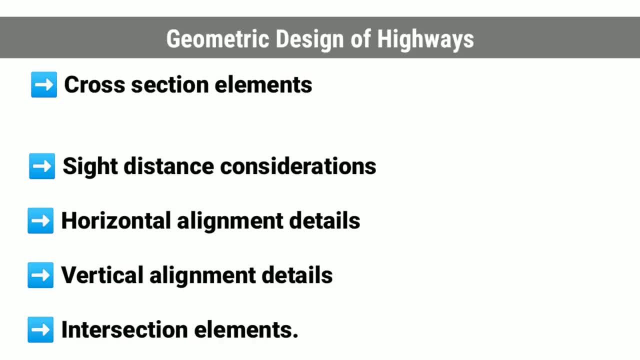 That is, cross-section elements, side distance considerations, horizontal alignments and vertical alignments. The vertical alignment details intersection elements. Under cross-section elements, the considerations for width of pavement formation and land, the surface characteristics and cross slope of pavement are included. The side: 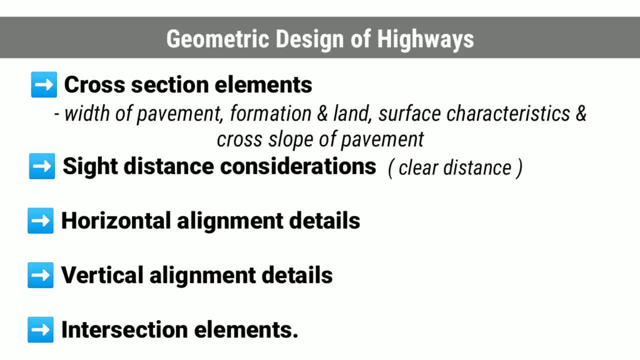 distance or clear distance visible ahead of your driver at horizontal and vertical curves and at intersection elements. The cross section elements are the rectangularお road either They are one to all 형 Break Point's. و angle is not the boundary point, It is the central line At the intersection. 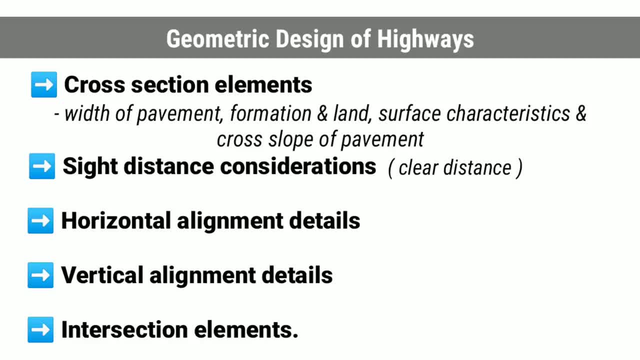 there is a crossed standing line at the intersection and stroll characters are blessing points of parking law. The intersection elements are transitions and vad Tools. Kanchan's provided on the horizontal curve In order to introduce centrifugal force and the super elevation. gradually, transition curves are introduced between the straight and circular. 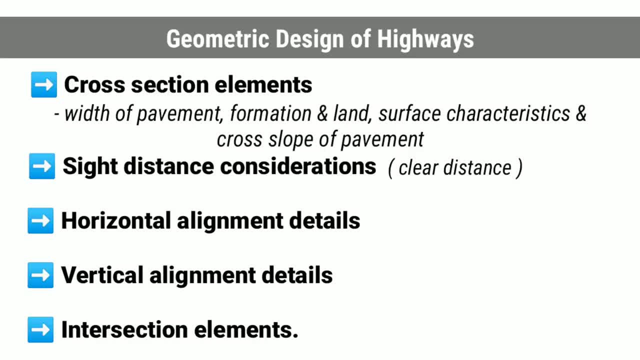 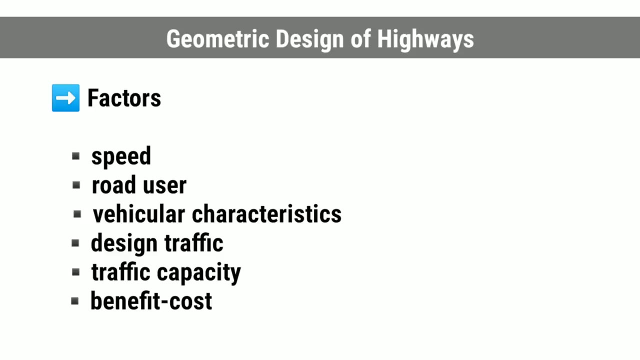 curves, The gradients and vertical curves are introduced on the vertical alignment of a highway. Design of road intersections with futures for safe and efficient traffic movement of vehicles need educate knowledge of traffic engineering. And here we see the factors which control the geometric design requirements are speed, road user and vehicular characteristics. 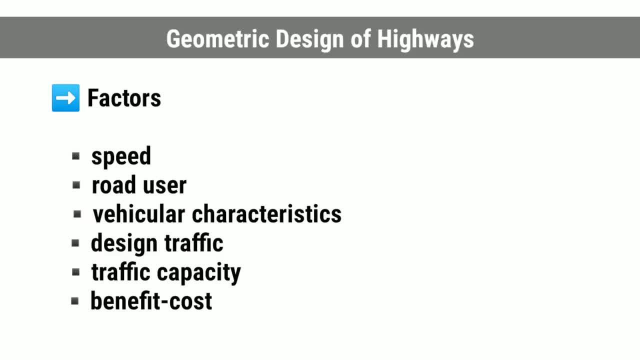 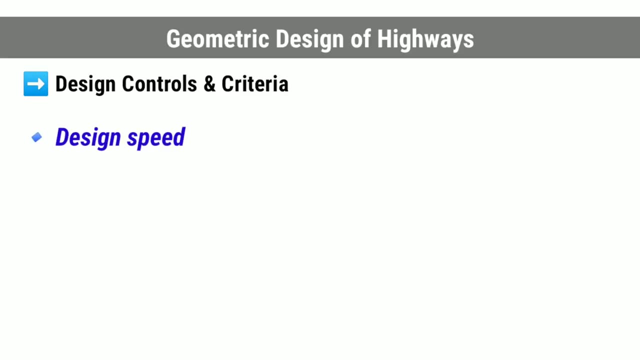 design, traffic, traffic capacity and benefit cost considerations. The geometric design of highways depends on several design factors. The important factors which control the geometric elements are design speed. First, let's see the design speed. The design speed is the most important factor controlling the geometric design elements of highways design. 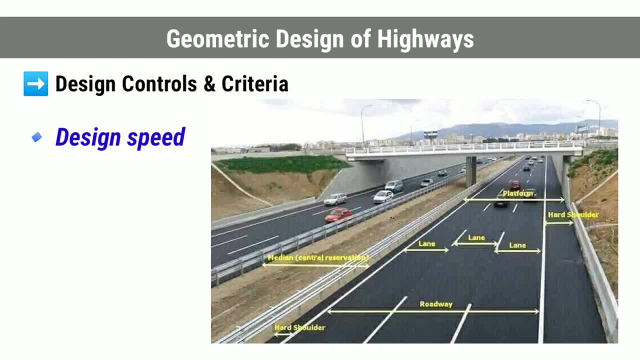 of almost every geometry design element of your road is dependent on the design speed. For example, the requirements of the pavement surface surface characteristics, the The cross-section elements of the road, such as width and clearance requirements, the side distance requirements are decided based on the design speed of the road. 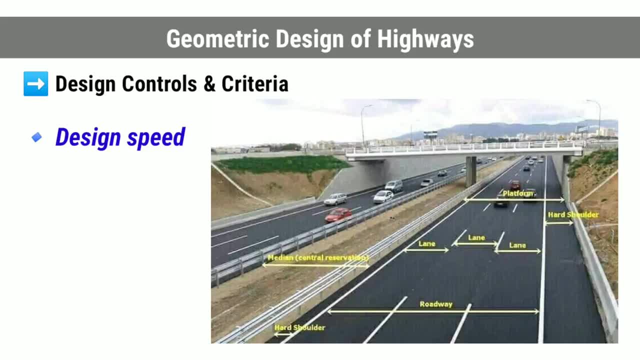 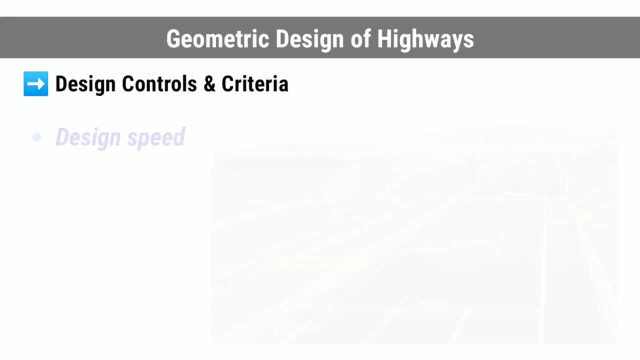 Also the horizontal elements, such as radius of curve, super elevation, transition curve length, and vertical alignment, such as gradient length of summit and valley curves, depends mainly on the design. speed on the road. And next one is topography or terrain. The topography or the terrain conditions influence the geometric design of highway significantly. 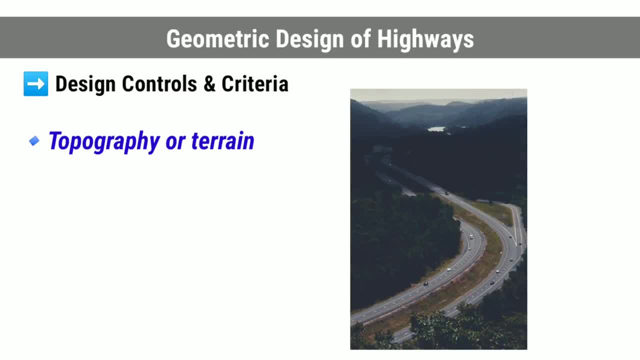 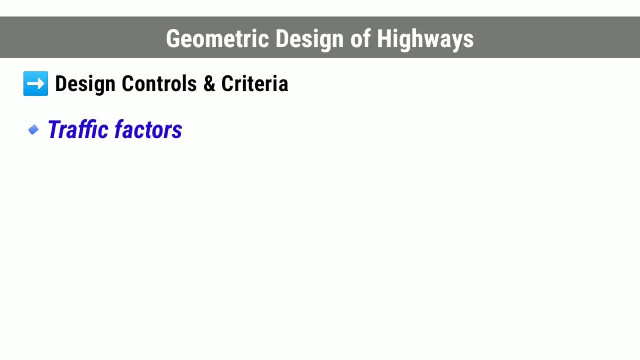 The terrains are classified, based on the general slope of the country across the alignment, as plain, rolling, mountainous and steep terrains, as given. And next we see about the traffic factors. The traffic factors associated with the traffic geometric design of roads are the vehicular characteristics and human characteristics of road users. 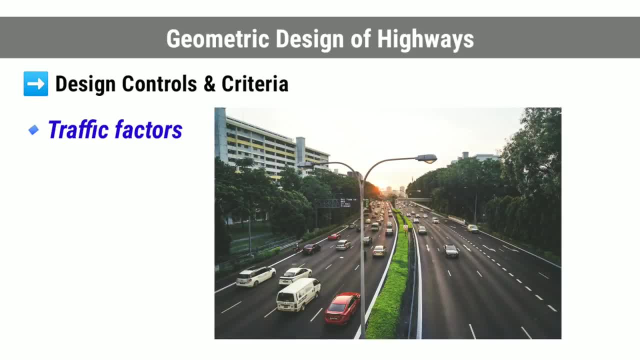 The different vehicle classes, such as passenger cars, buses, trucks, motorcycles and various other types of non-monetarized vehicles, are different speed and acceleration characteristics, Apart from having different dimensions and weights. the important human factors which affect the traffic behavior include the physical and mental and psychological factors of drivers and pedestrians. 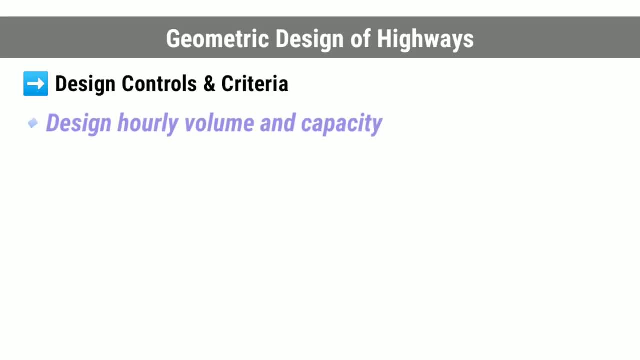 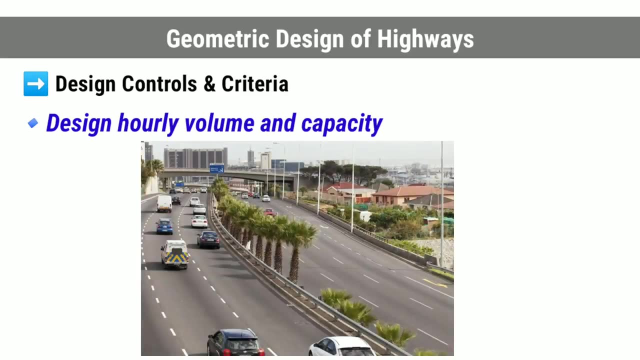 These all comes under traffic factors And next we see about design, early volume and capacity. The traffic flow or volume keeps fluctuating From a low value during setting of peak hours to the high flow during the peak hours. it will be uneconomical to design the roadway facilities for the peak traffic flow or the highest or early traffic volume.